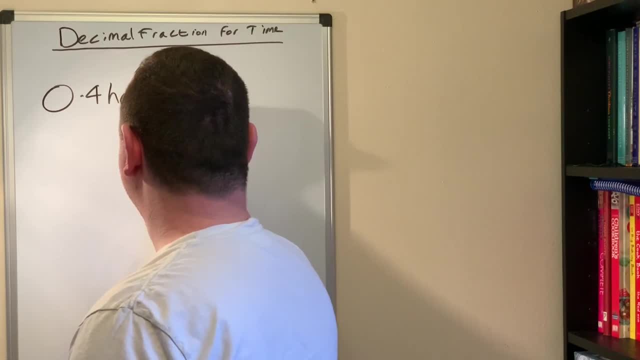 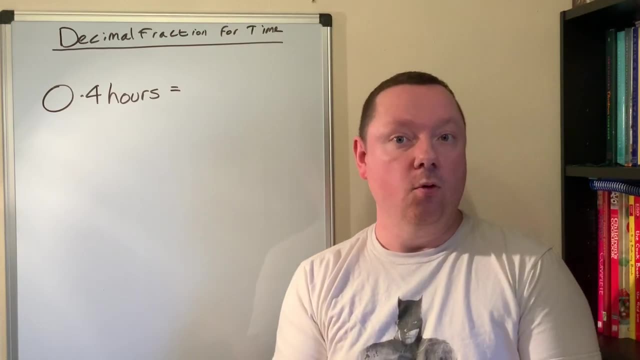 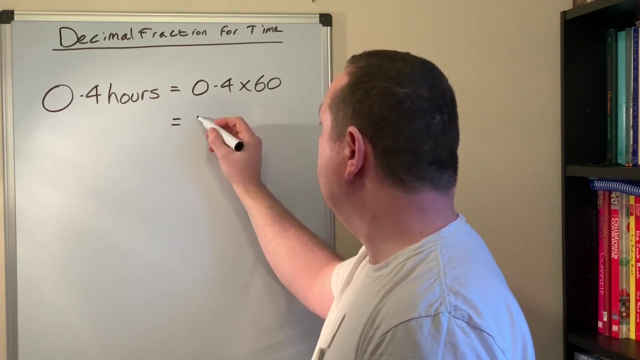 hours and I want to change that to minutes Well before. we're divided by 60, so we'll do the opposite. if we're going the other way, times by 60. So I just need to do 0.4 times 60, which would give 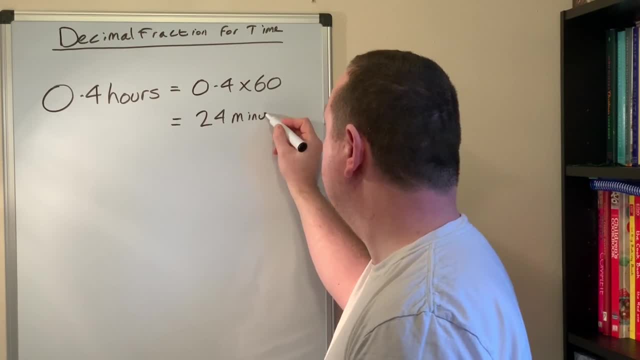 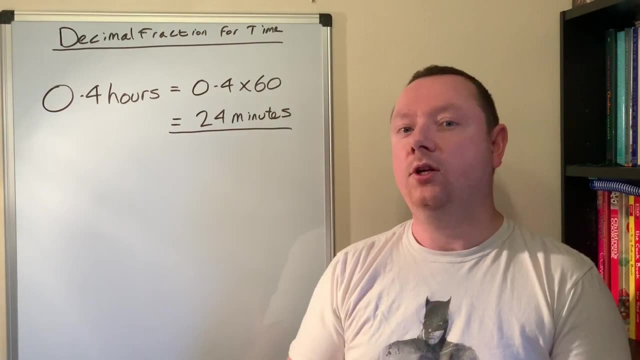 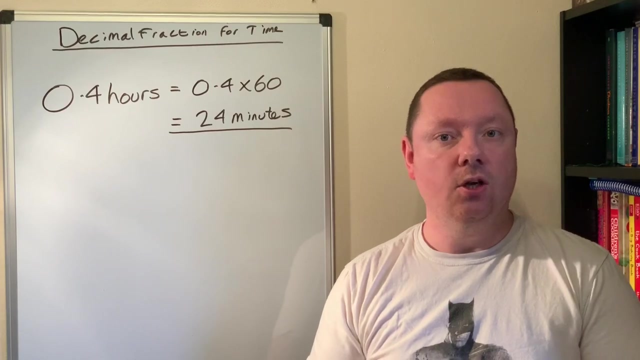 me 24.. minutes, And it will be in the context of the question. you'll know whether you need to leave your answer as hours and minutes, which means you'll have to do it this way, or whether you'll be happy enough to leave your answer as just a decimal hour. 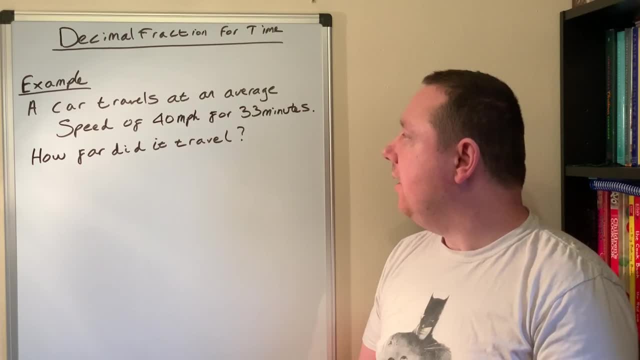 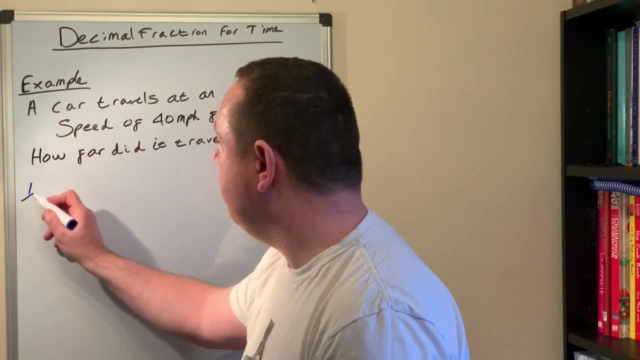 So example: a car travels at an average speed of 40 miles per hour, or 33 minutes. How far did it travel? So step one is the same as in previous examples, where you've got two different things: you've got hours for the miles per hour, you've got minutes for the time. 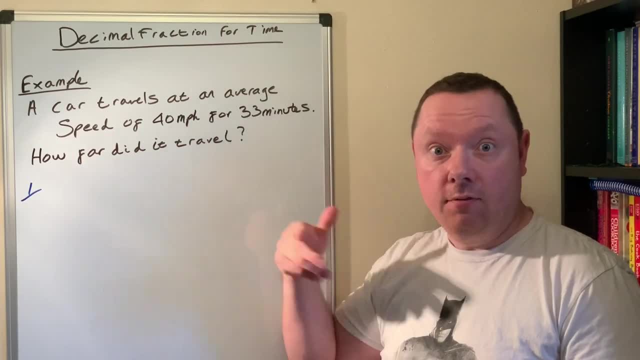 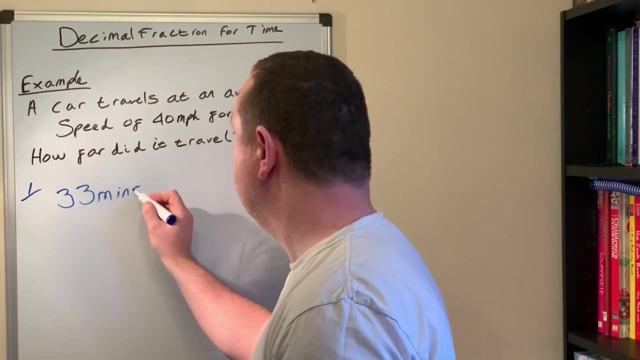 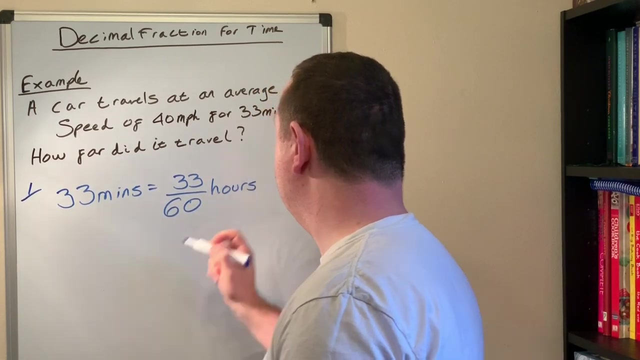 so you're always changing minutes to a bit of an hour, a fraction of an hour or a decimal. So I've got 33 minutes. so that's 33 out of 60 hours. but you should notice, when you look at 33 out of 60 it's not a very. 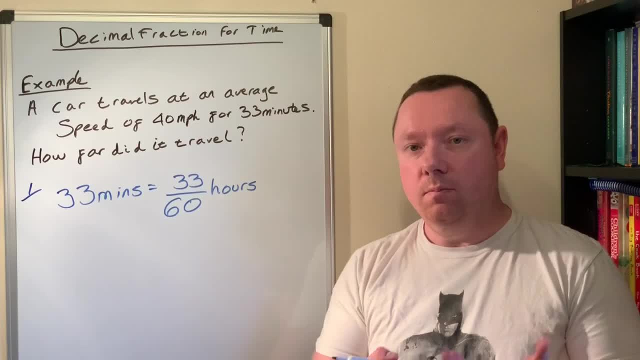 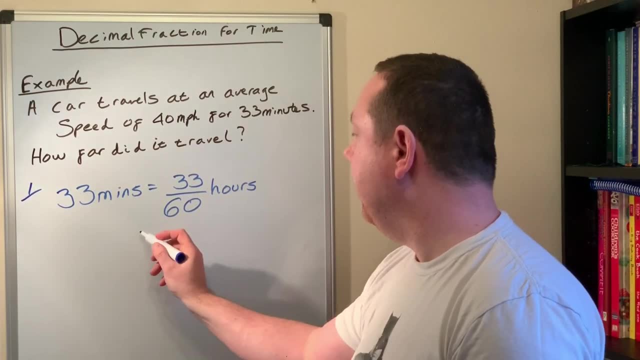 convenient fraction. you can simplify it a little bit. but if you're using a calculator, bit off straight away just go straight in to change it to a decimal. so we're going to just do that. if you can't simplify it to a nice small fraction like a half a quarter, use a calculator. 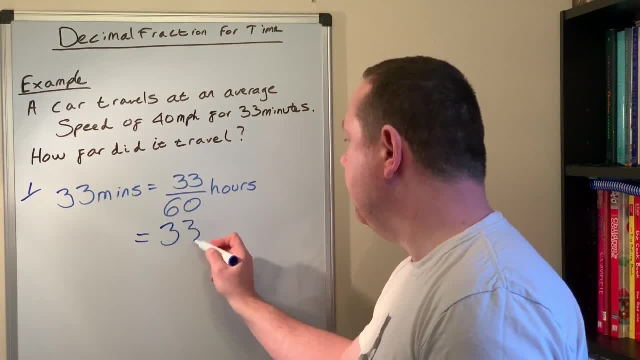 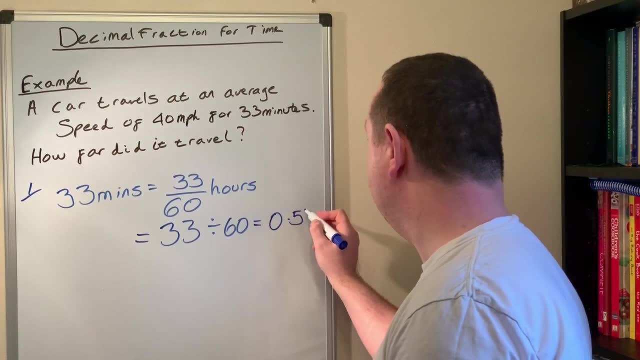 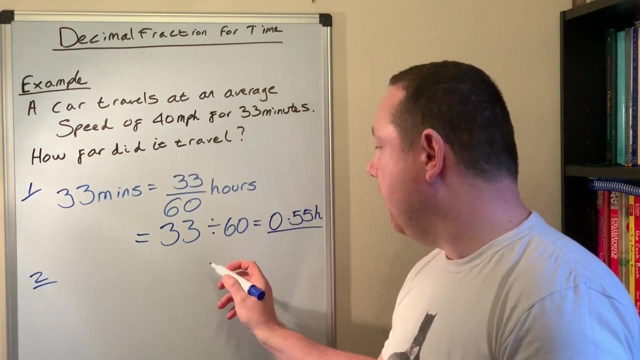 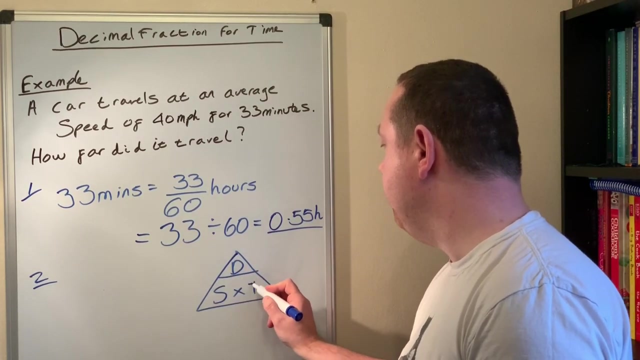 change it to a decimal. i need to do 33 divided by 60, 0.55 hours. so step two: we use a speed distance time. so we need a triangle distance on the top over speed times time. i'm trying to look at how far i traveled, so i covered distance up and it says do speed times time. so i write down my 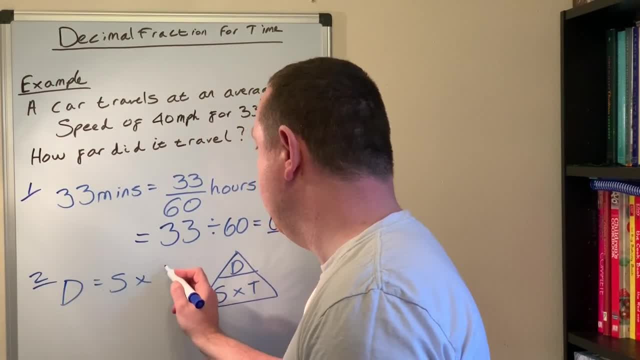 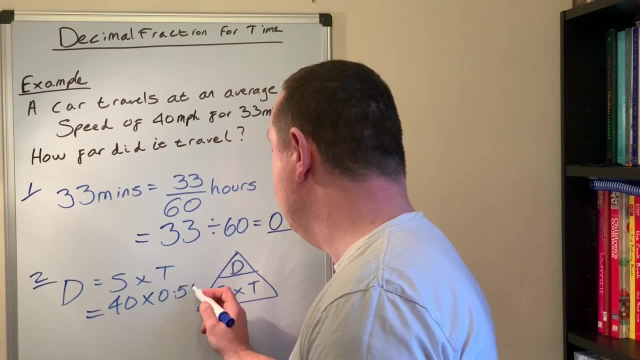 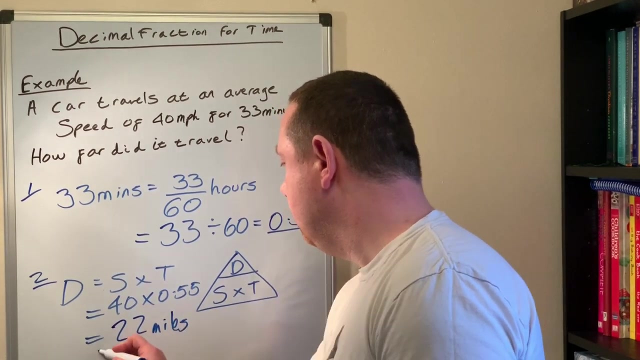 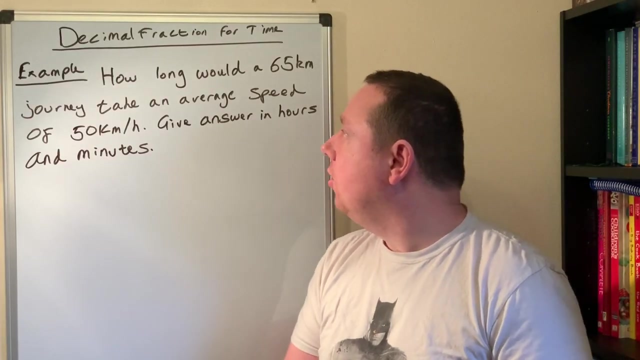 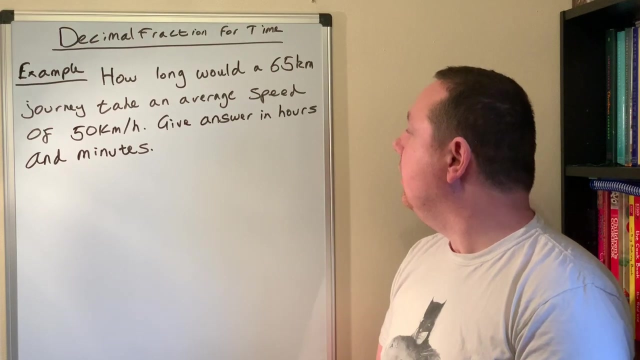 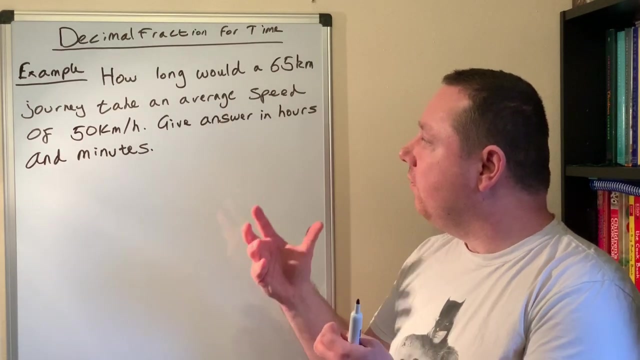 formula: distance equals speed times. time speed is 40, the time is 0.55, now miles. let's look at another example. so example: how long would a 65 kilometer journey take at an average speed of 50 kilometers per hour? and if they give you an answer in hours and minutes? so there's no conversion to do yet. 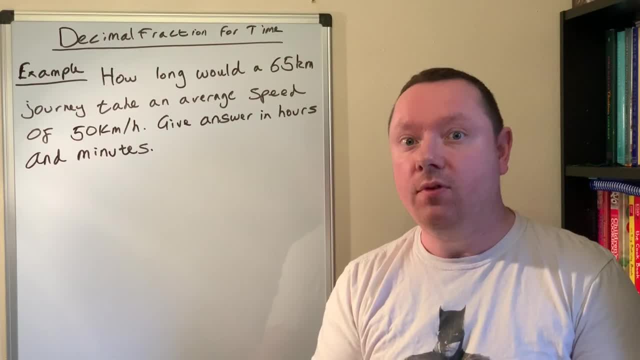 because i've not worked out the time. so if you've not got the time to convert, you don't have to work out the time. so if you've not got the time to convert, you don't have to work out the time. you need to wait to the end to do that. so step one in this case, 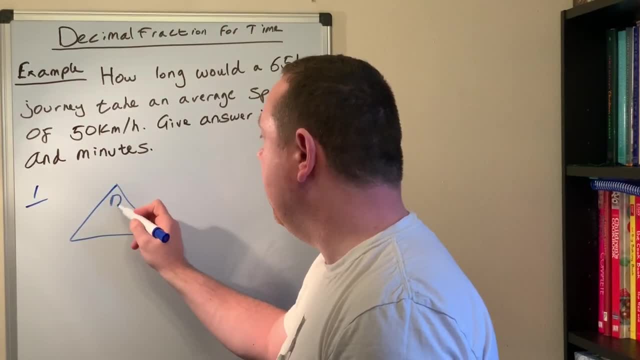 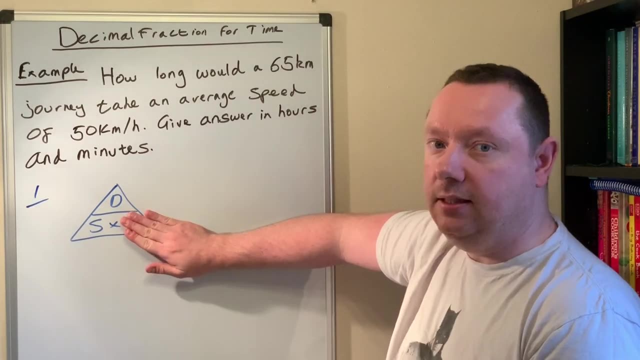 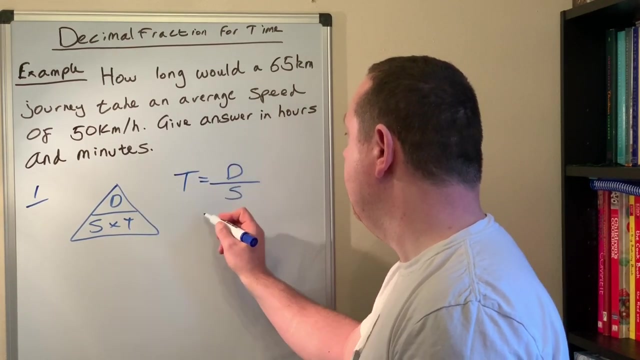 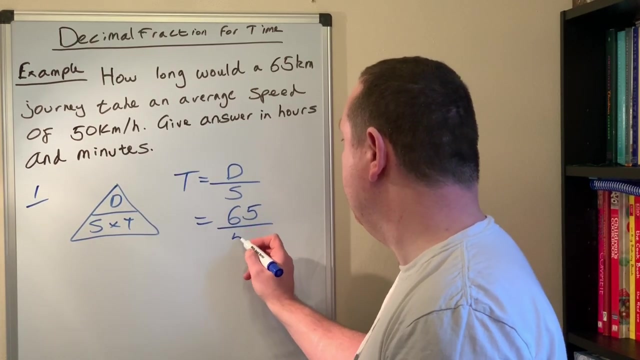 is just to draw my distance. speed time triangle. i'm looking for the time so i covered up the t and it says d over s, so i can write: the t equals d divided by s, the distance is 65 kilometers and the speed is 50 kilometers per hour. 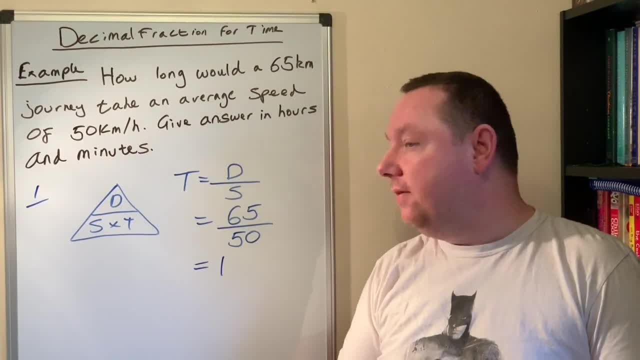 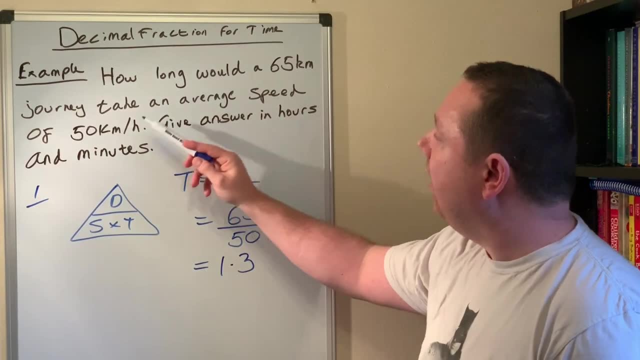 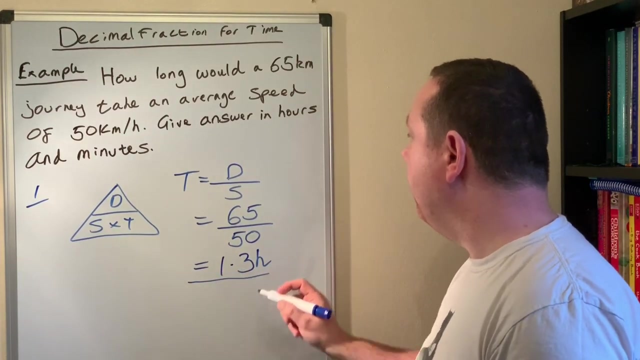 65 divided by 50, which is 1.3. now the units on this at the moment is hours, because the speed was kilometers per hour. so it's 1.3 hours. but if i look back at my question it says: give answer in hours and 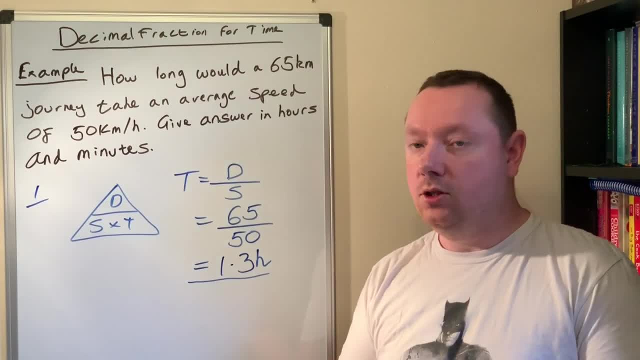 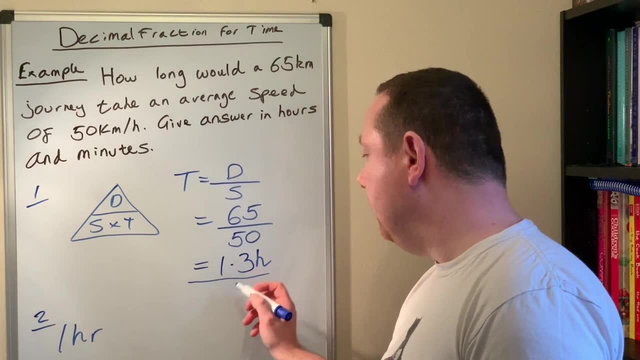 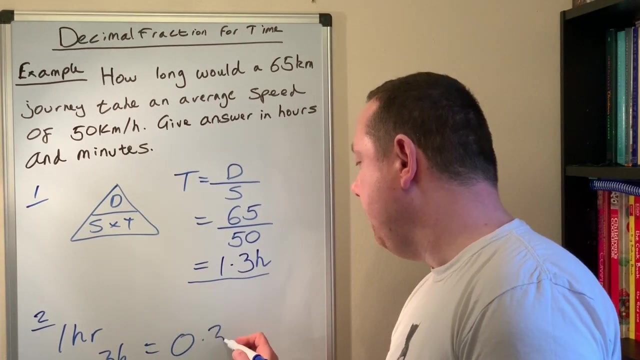 minutes. so we'll have to change this 1.3 to hours and minutes. okay, so i've already got step two. i've already got one hour, but i've got the 0.3. so the 0.3 i need to change to minutes. so i times that by 60, 0.3 times 60. 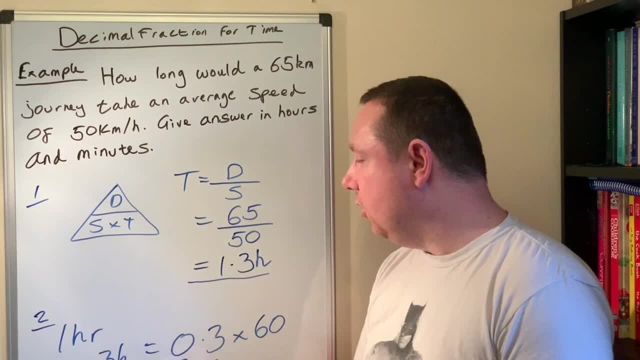 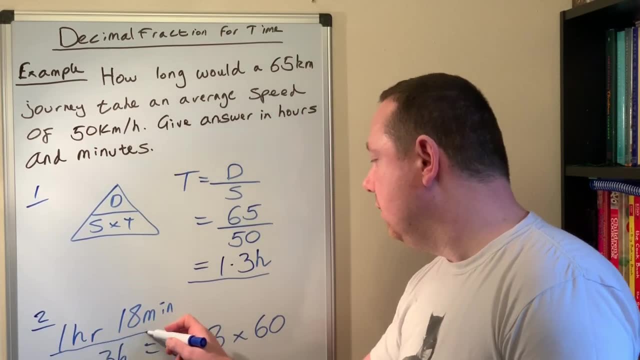 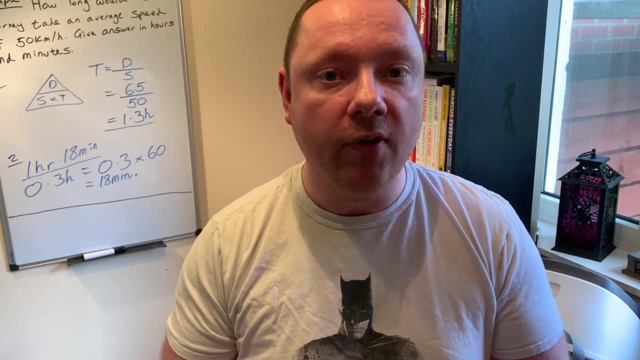 which is 18 minutes. now my 1.3 hours is one hour 18 minutes and that's my final answer. mr clown here, thanks for watching that video on changing minutes to decimal fractions of an hour. hopefully you found that useful and you're now able to do all the problems that you need to do in relation to the distance, speed and time formula. 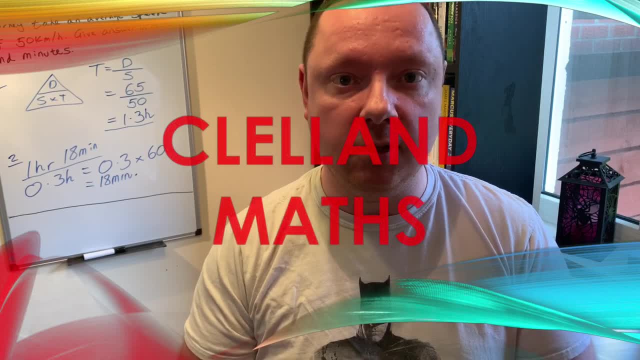 if you need any further, help check the links in the description, and please remember to subscribe.